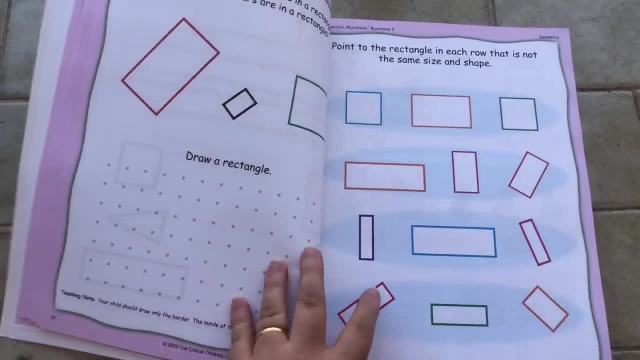 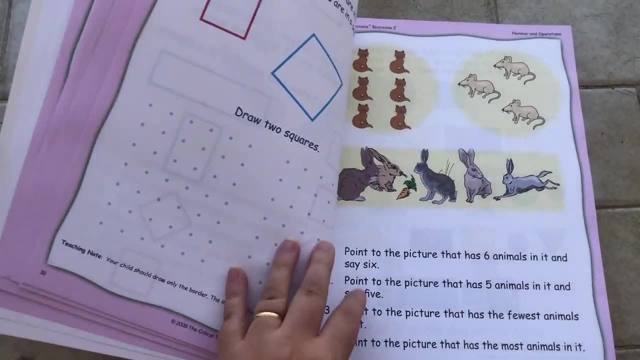 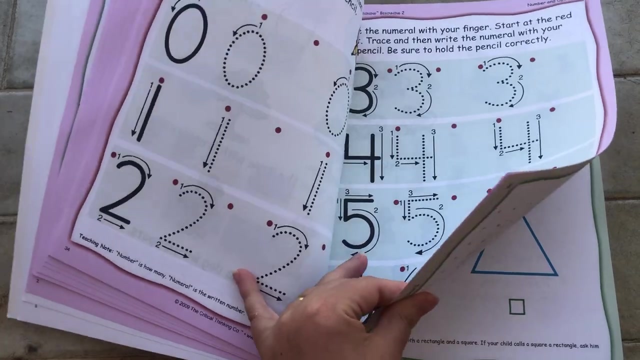 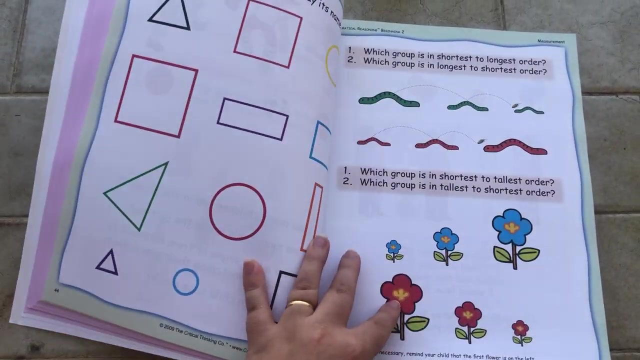 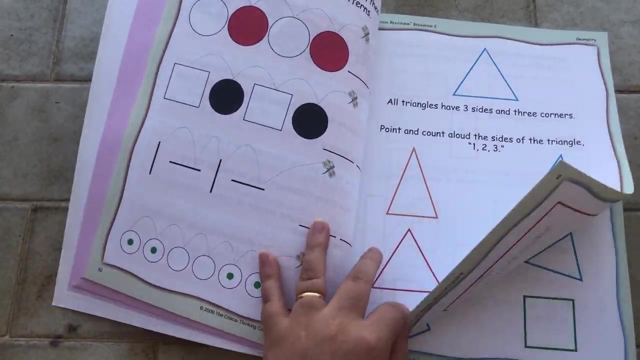 beautiful. I originally got it because we've done an ever more workbook. I'll give, I'll give you the tags. But that book is pre-K and I don't think she's ready to move on level K because she's only three and a half. So the thing is she's quite good at numbers. 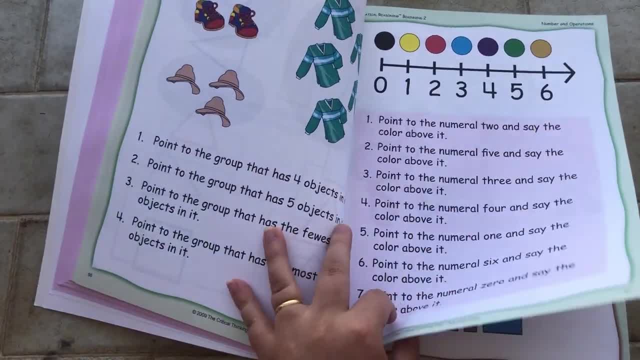 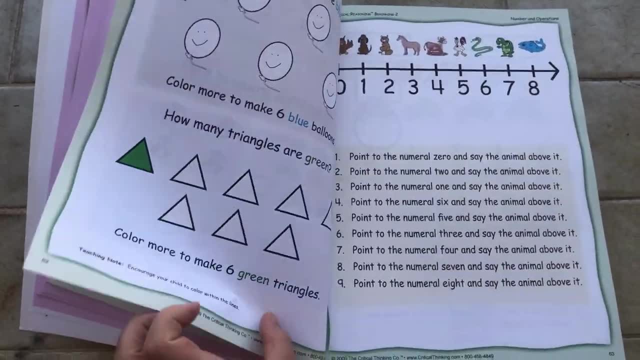 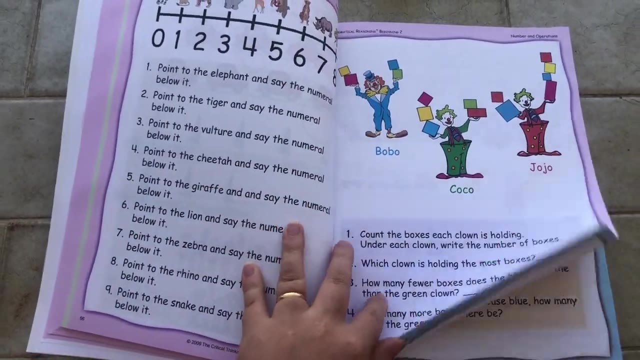 and some addition and she can read the numbers, so she can sort of write, but not so well. But, as in this sort of exercises, she's great, But she doesn't do that well with reasoning skills. So for instance, she's not good at finding that different object where they give. 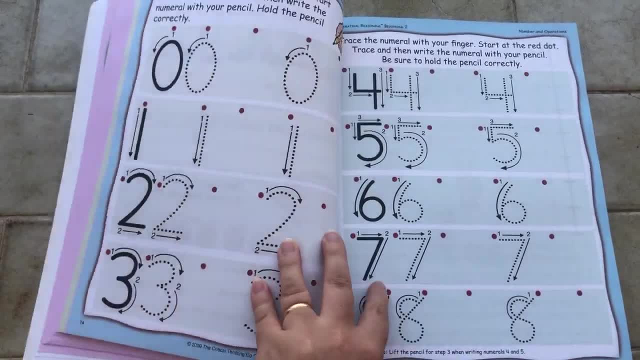 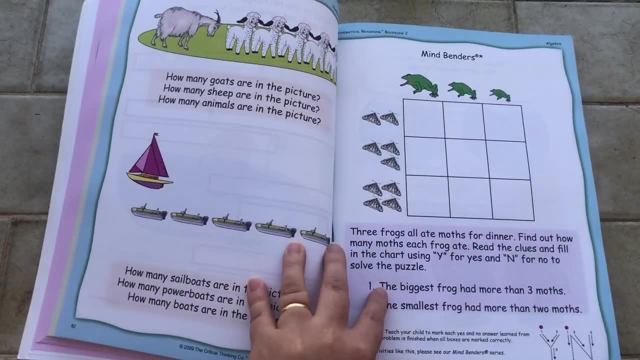 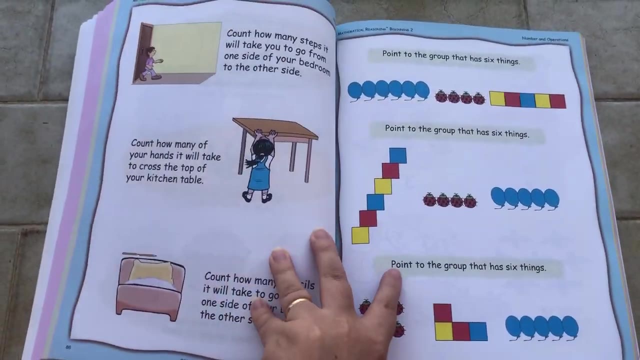 you- I don't know- four pictures and you need to find the one that is different, and stuff like that. So I thought that she needs slightly less classic math and more thinking skills like this sort of stuff. So instead of going from pre-K to K, she's going to K again, but 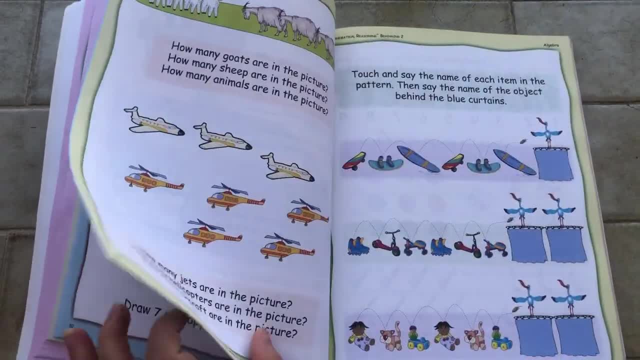 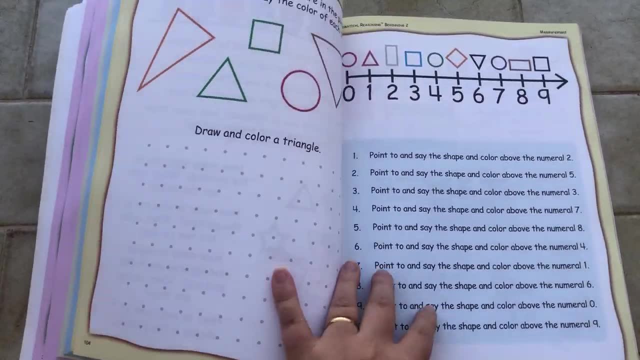 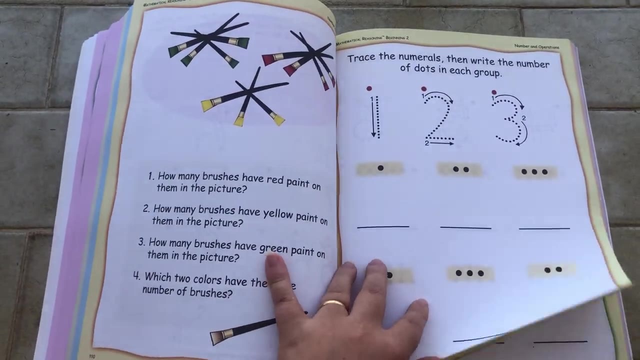 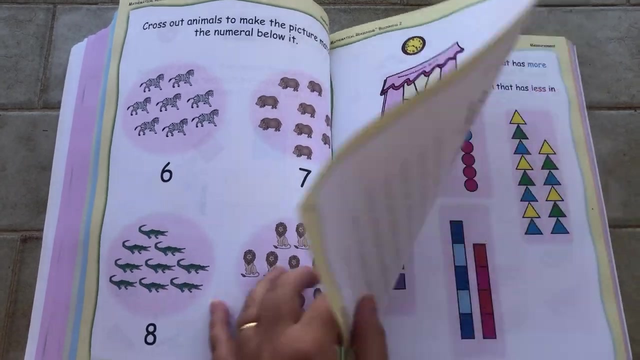 with more thinking and more writing. So I think this book was perfect for this. I also was lucky because I found it on Amazon. It was technically second hand but actually it had been returned, So it was new but returned to the shop. So it's perfect on the inside: no writing, no scribbling, no anything. It 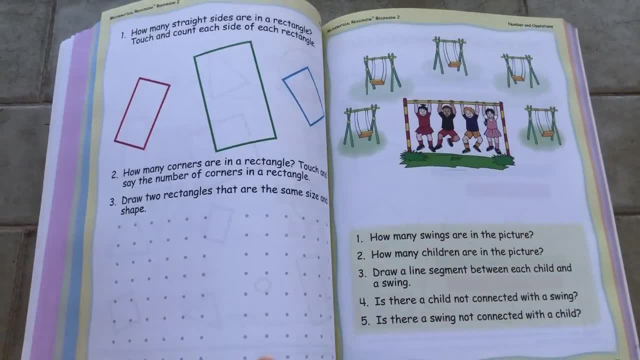 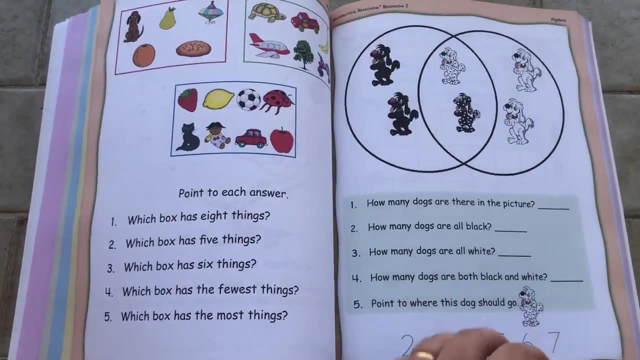 just has slightly damaged parts. It's covered, but nothing bad. Like you can. it's worn, if that makes sense. So it's been traveling around. It makes sense that it's not perfect, but hey, we saved some back, so that's good. 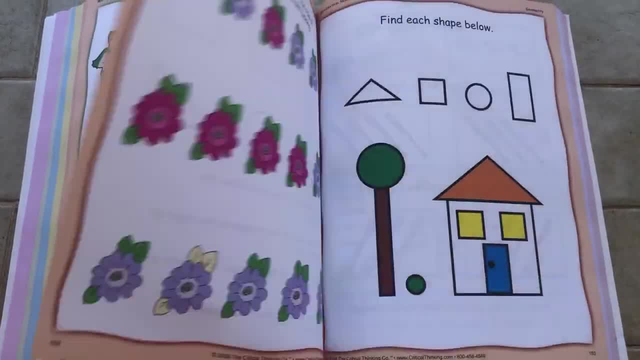 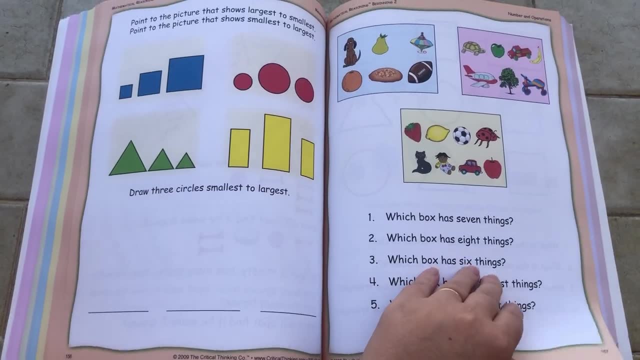 And about the drawings. I really don't like this. I don't know. My daughter seems to like it, so that's not an issue, But I think this book with, except for this one, I don't know, I don't know, I don't know. 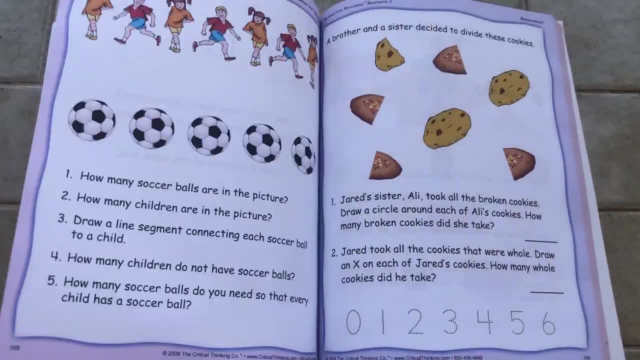 But I think this book with, except for this one, I don't know, I don't know, I don't know. I think this book with, except for this one, I don't know. But I think this book with exactly the same content but renewed illustrations, would be amazing, Would be able to compete. 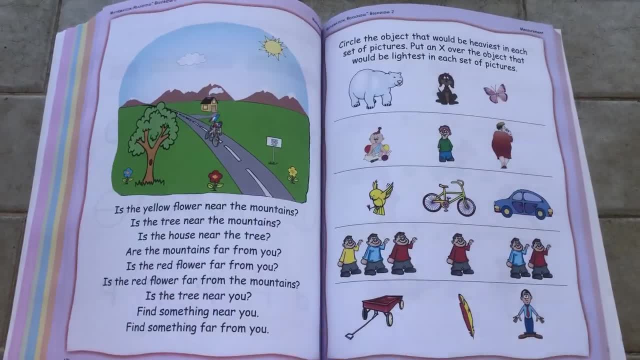 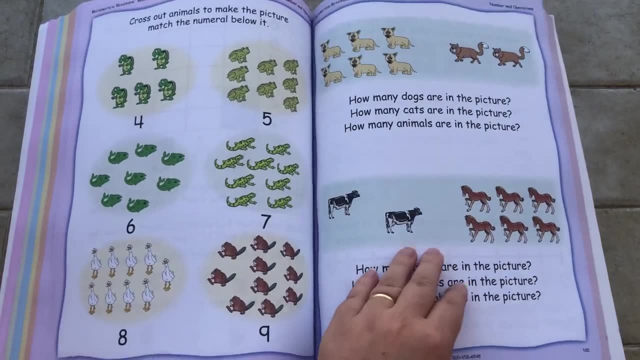 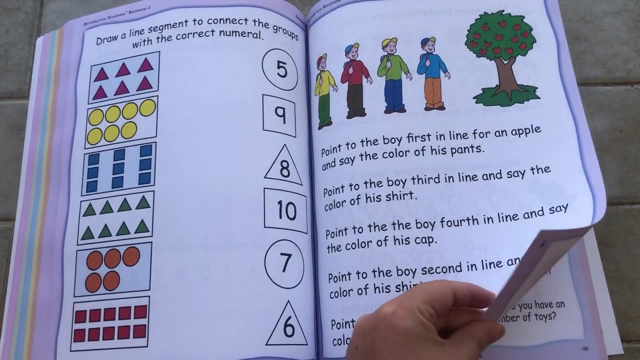 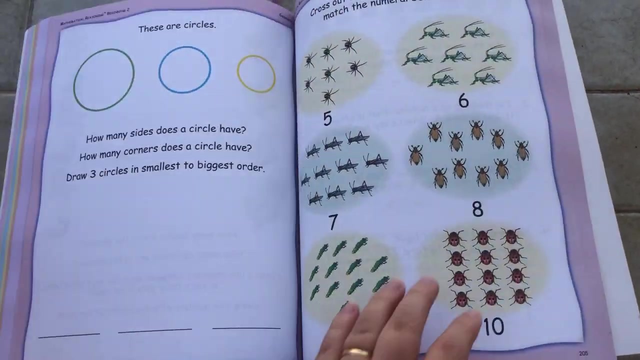 with some of the big companies out there. I like this design. Yeah, I think it goes to. It does numbers up until 12 or 13,. we'll check it later. Hold on, I don't want the book to close. 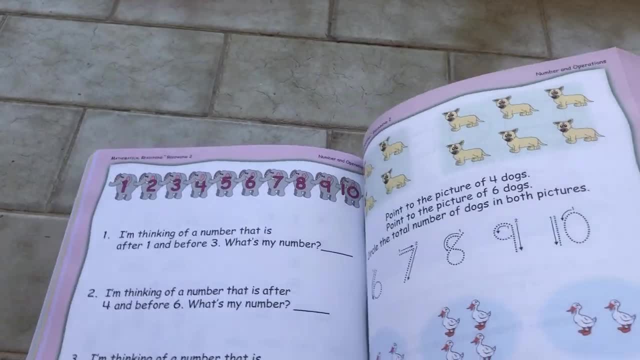 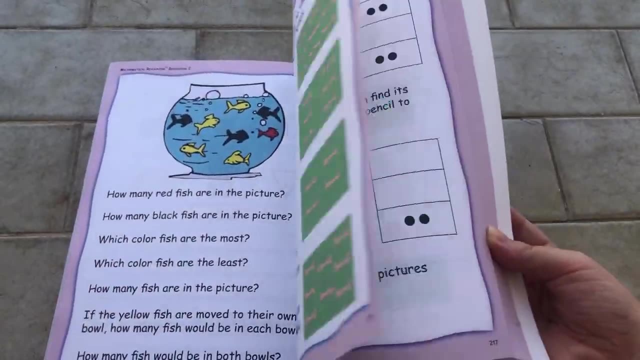 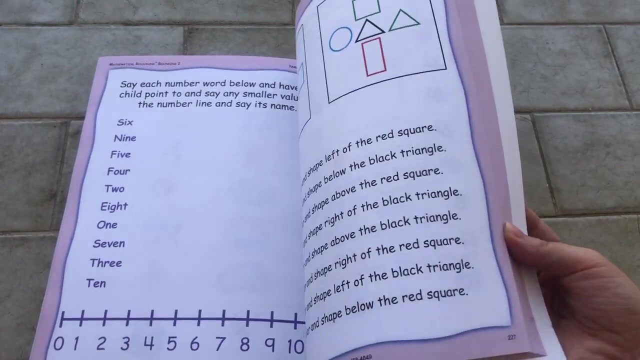 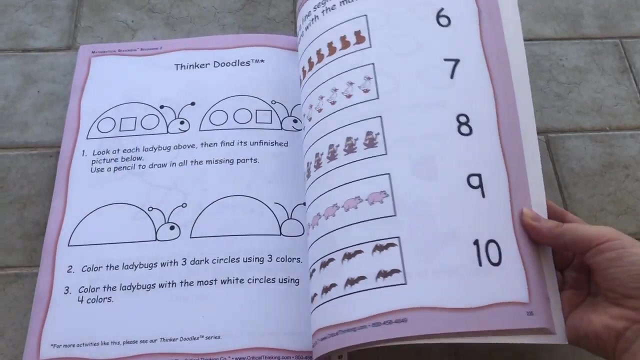 There we go. I'm going slightly faster because the video is already almost 5 minutes. Something I noticed before is this book doesn't have an answer key. I mean it's for 4 year olds, so we're supposed to know what's going on. 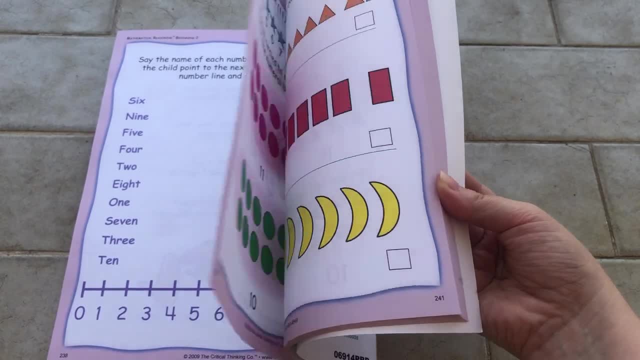 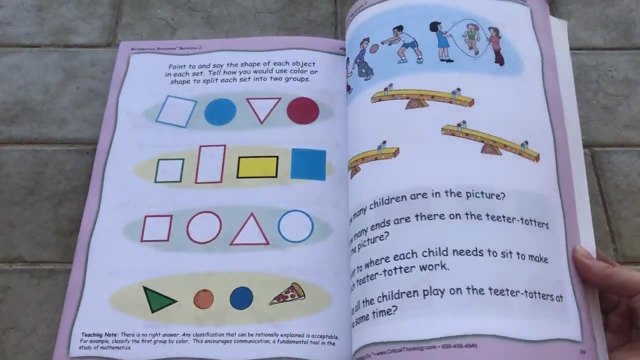 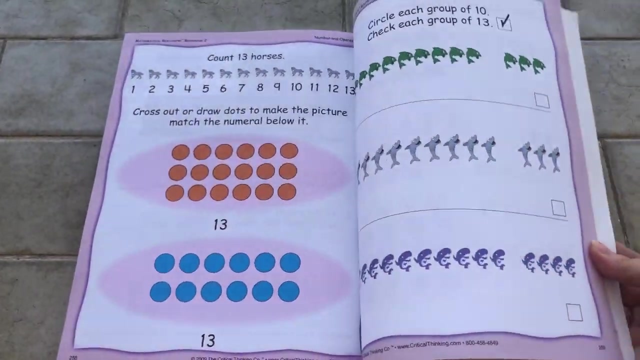 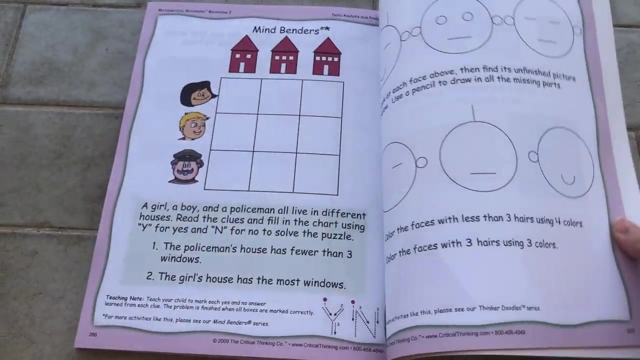 but I don't know if it's the same for all the books from this particular publisher or if later on, when everything starts getting more difficult, there will be an answer key. Lots of exercises on counting and the number line. There's some logic exercises like this one. 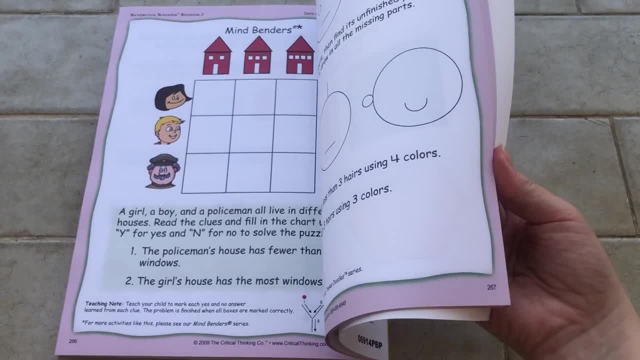 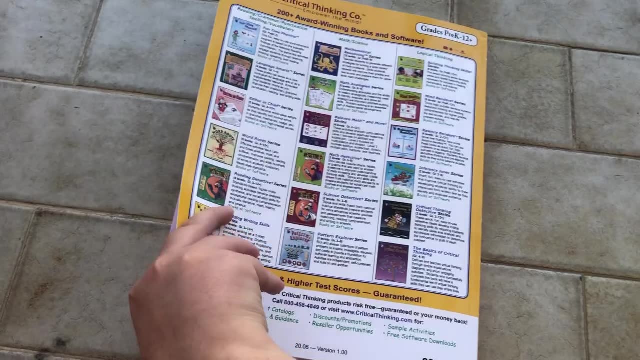 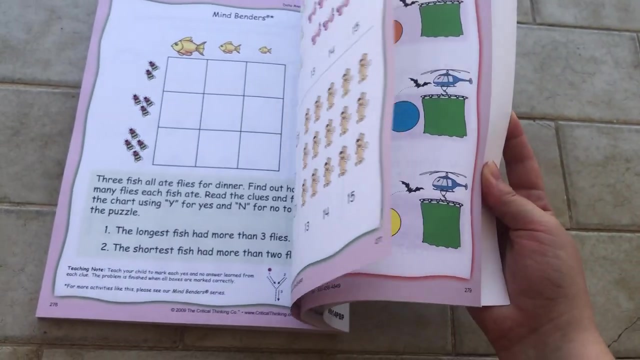 which I find super interesting: Some drawing symmetry. Overall, obviously, Ah, it goes to 15, I thought it went only to 14.. Overall, I find it a very good investment. I only paid, like I think it was 25 bucks for it because I got it used. 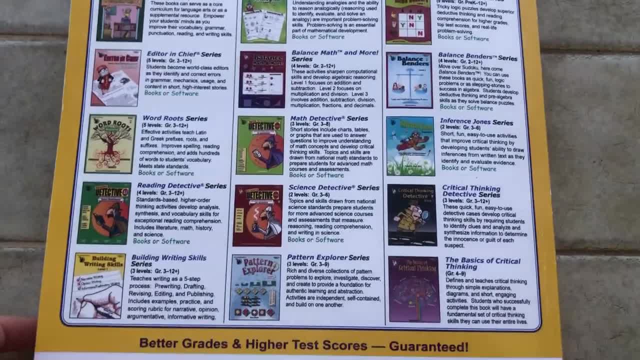 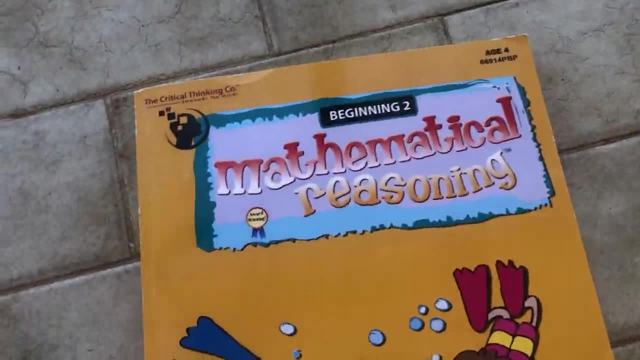 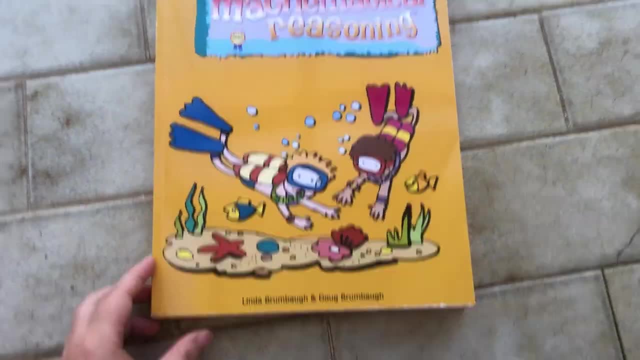 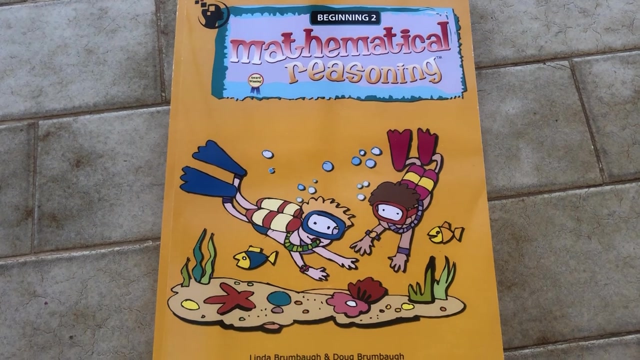 But it's gorgeous. Here's everything They have And, yeah, what I told you about it not being perfect- you see These corners, that- But besides that, it's basically a new book, So I'm super, super happy with this and looking forward to start using it.